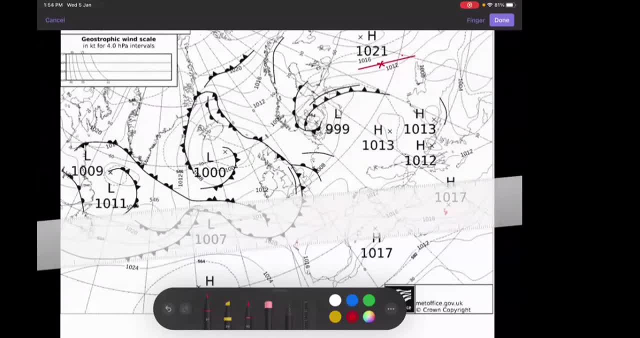 Yes, sir, Now you're getting confused. There is no pressure, gradient wind, and all that In this case, because he's asking you on that spot. He's asking you on that spot Now I am thinking that where the wind will be going. 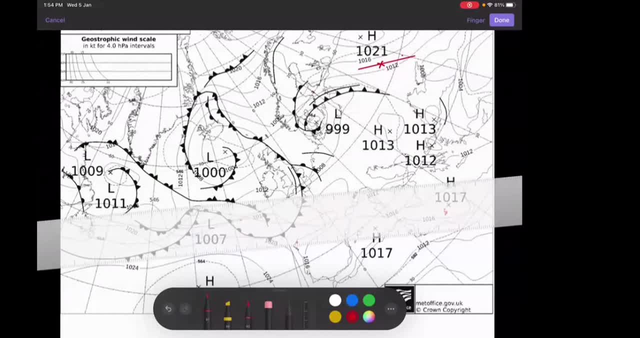 Yes, Correct, Yeah, correct, Correct, Where the wind is coming from. So basically now I am getting confused Whether the wind is here Or from the other side. Yes, Or from the other side- Yes. So what do you think? 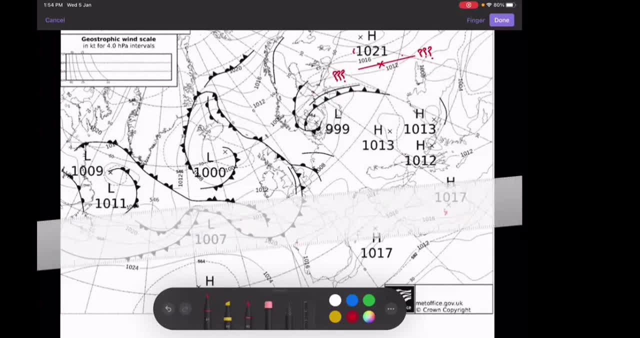 So I start looking at the What is this isobar. What is this isobar? 1, 0, 2, 1.. 1, 0, 1, 6.. 1, 0.. 1, 6.. 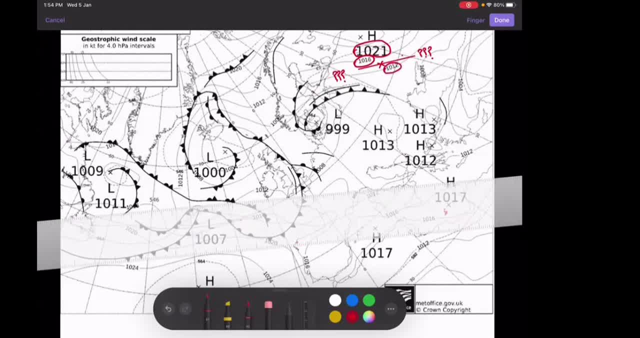 What is the next one? 1, 0,, 1, 2.. Then after that you have no isobar, But you know there is a low pressure also here. Yes, Correct, So according to the Bayer-Ballet's law, you are facing the wind. 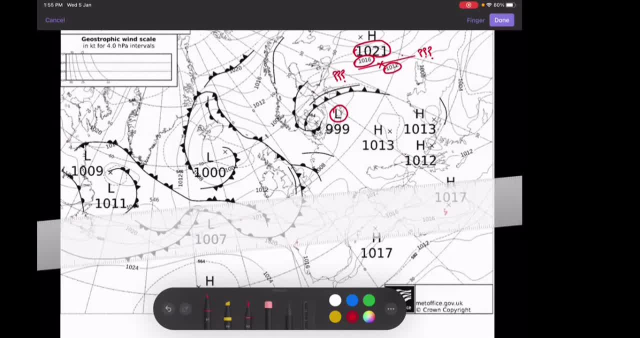 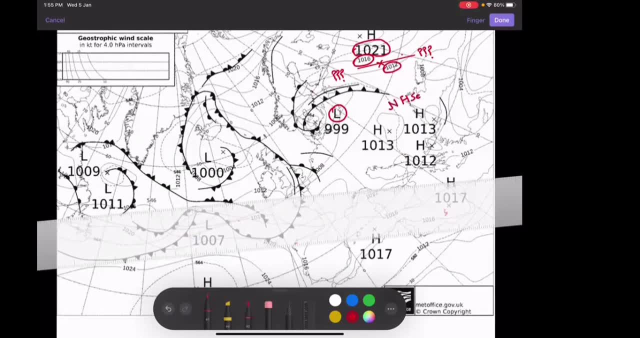 Right And the low pressure lies on your right-hand side. If you are in what? sphere? Northern Hemisphere, Northern Hemisphere, Northern Hemisphere, Isn't it Correct? Yes, Correct. So if you are in the Northern Hemisphere, then what will happen, Jitu? 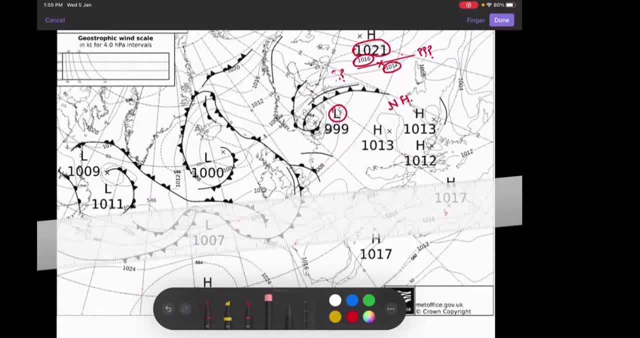 From where the wind is coming. now Tell me, You are facing the wind, isn't it? If the low pressure is on your right side, you are facing the wind. So where is the wind coming from? Where is the wind coming from? 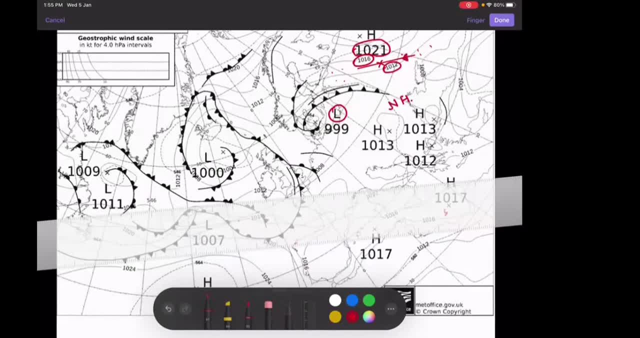 From this direction, isn't it Correct? Yes, There is no flare yet, sir. Huh, There is no flare, sir. Okay, Okay, Okay, Okay Again. If you don't understand, it's okay. This is a parallel line, correct. 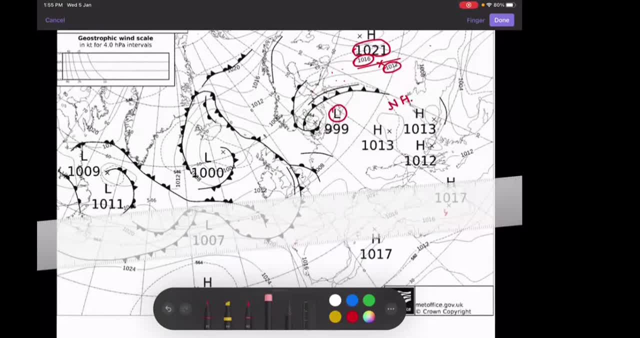 Correct sir. Did you understand that or no? I understood Parallel line here. What is this pressure over here? 1, 0, 2, 1.. 1, 0, 2, 1, yeah, yeah. 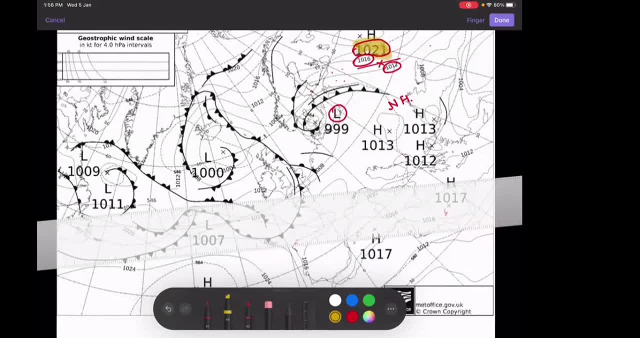 This pressure is 1, 0, 2, 1, isn't it? Yes, Then you have got 1, 0, 1, 6, isn't it? The pressure is dropping 1, 0, 1, 2,, isn't it? 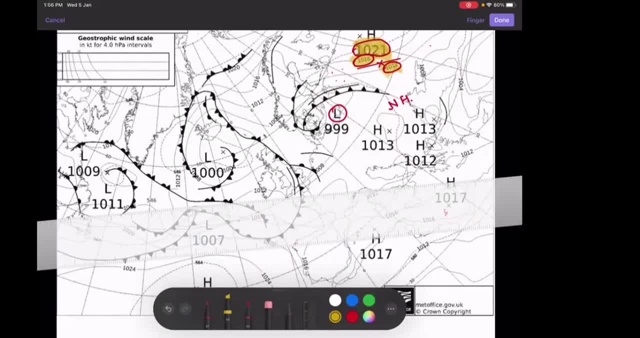 Yes, So where is the low pressure? Low pressure is on the right, isn't it Right? And it is very significant that low pressure is, of course, the low is, you know, continuously low: 1, 0,, 2,, 1, 1,, 0,, 1,, 6,, this, and there is a low there, also on your right. 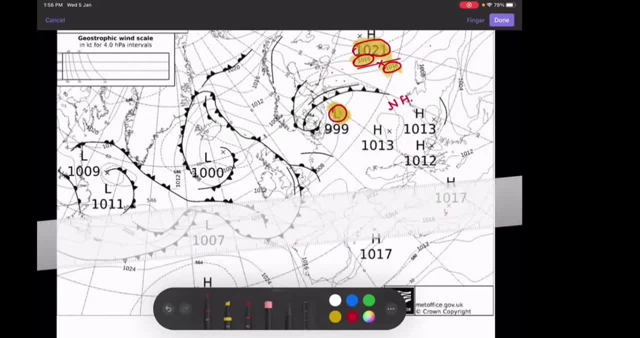 So wind will definitely come. from which direction You are facing the wind? If you are here, Jithu, Yeah, If you are there, if you are there, if you are standing there, you are facing the wind, isn't it? 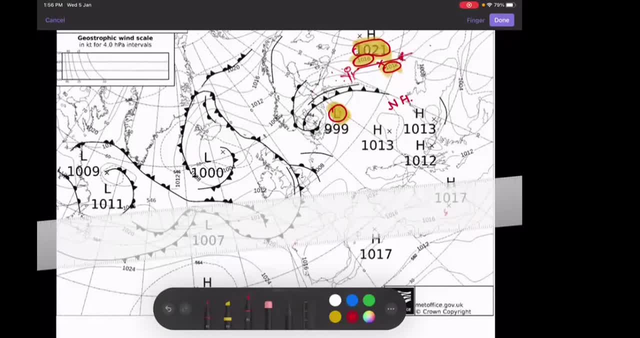 So wind is coming from this one, Then only you can face: Yeah, So now, what is this direction? So, to measure this direction again, now you know that it is coming from there. Yeah, Correct. So what you do is you. 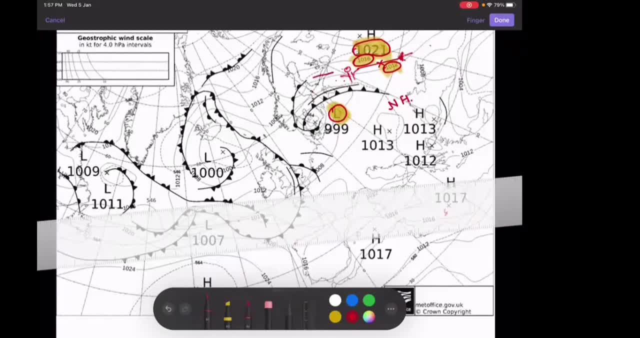 You, now you increase this line to here: Yeah, Correct, Okay, Then this is the latitude and the longitude you are talking about, isn't it Correct? Make And make the latitude like this: Yeah, Now, what is the wind now? 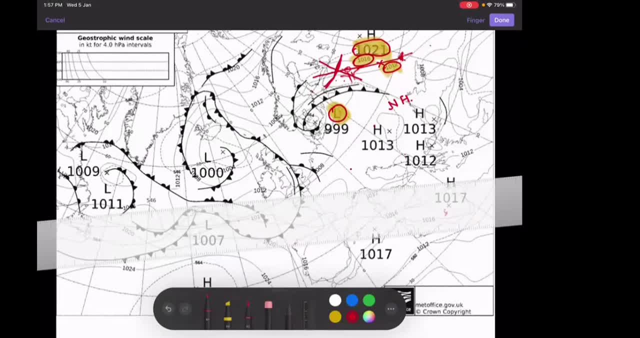 Tell me That is approximately south-easterly wind. South-easterly, Everybody get this, or not? Somebody said easterly, No It. Where is the north and south? You have to establish that also, my friend. Yes. 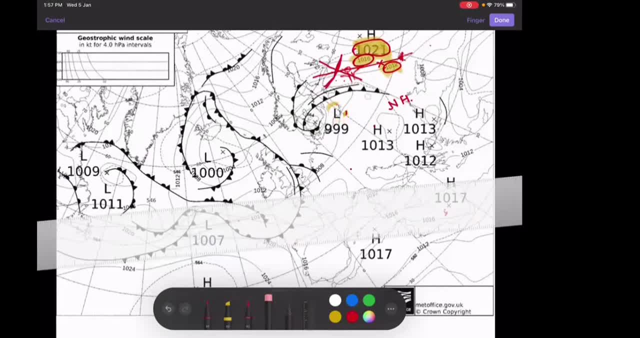 Understood or not Understood, sir? Understood: Everybody is with me, or no, Sir? this line is just parallel. Sir, this line is just parallel to the item right. So we need to draw the in-raft angle also, correct? 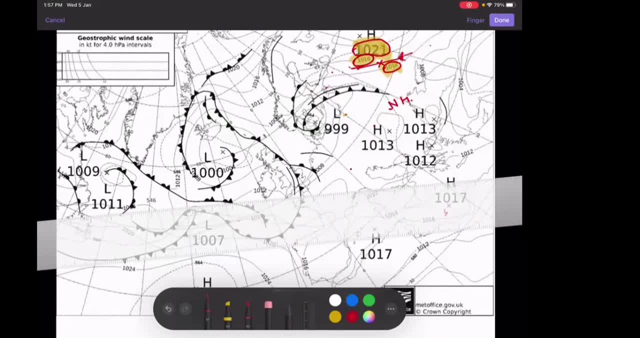 Yeah, That is See, that is correct. That is correct. Yes, You, That is correct. What I am saying is that You have a wind like this. Yes, of course, you will make some in-raft angle also. 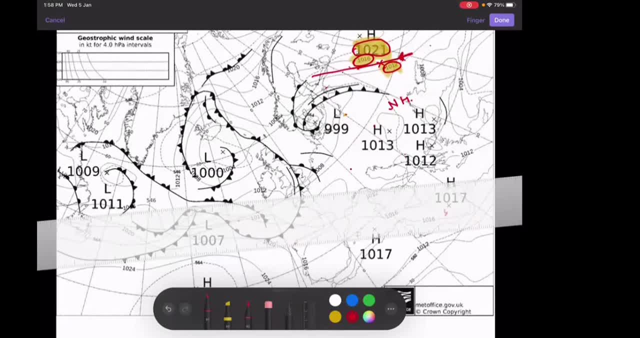 But it will still come in that quadrant of south-easterly only Because 20 degree will not change it that much. Okay, So if you make it like this, still it will be south-easterly, isn't it? Yes?